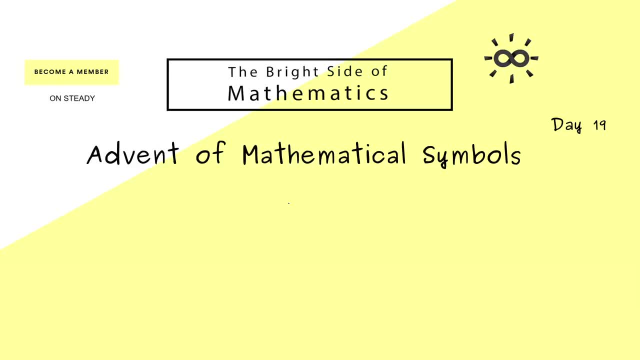 Hello and welcome. and the mathematical symbol of today is euler's phi function, denoted with a lowercase phi. It's also called euler's totient function and used in number theory. Therefore, the domain of the function is given by the positive integers. So we have the natural numbers n, starting with 1.. 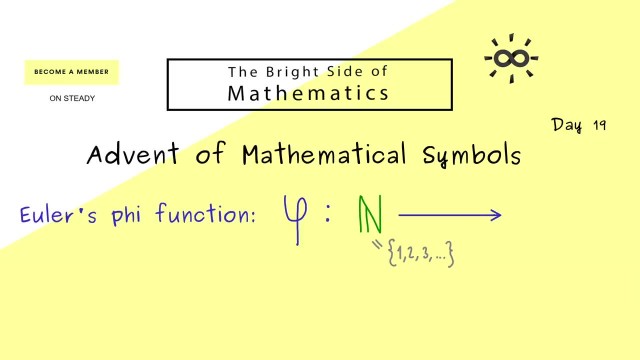 And also the codomain is given by the natural numbers. Now, of course, the question here should be: what is the definition of phi of n? And the short answer is that we simply have to count numbers with two properties. So let's use the letter a for the numbers we count and then explain the two properties. 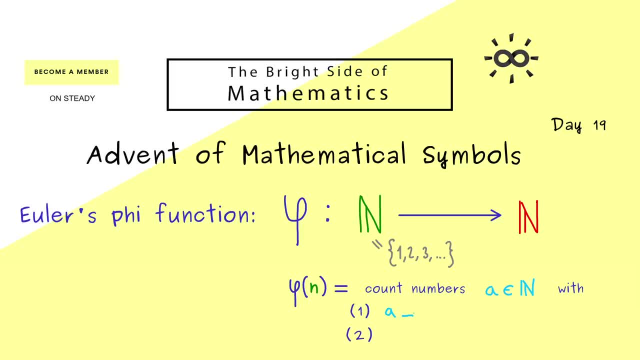 The first one is very simple. we only consider numbers that are less or equal than n. This means that the outcome of the phi function can never be greater than the input. Then the second property tells us that a and n don't have a single common divisor. 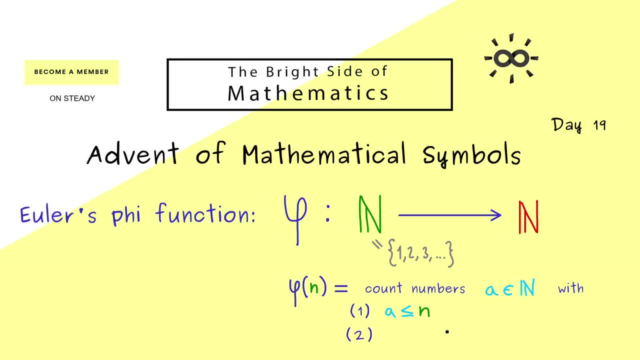 Of course, except 1, because 1 divides everything. Hence we can write this as the greatest common divisor, gcd of a and n is equal to 1.. In mathematics then we say that a and n are mutually prime. Now, if you have never seen the example of a and n, 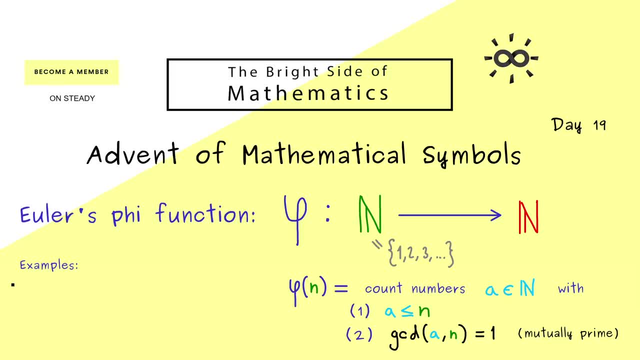 Then I think examples will help. For example, what is phi of 4?? Now, because of property 1, we already know. we only have to look at the numbers 1, 2, 3 and 4.. Of course, property 2 immediately tells us that the number itself- so 4 here- cannot be counted. 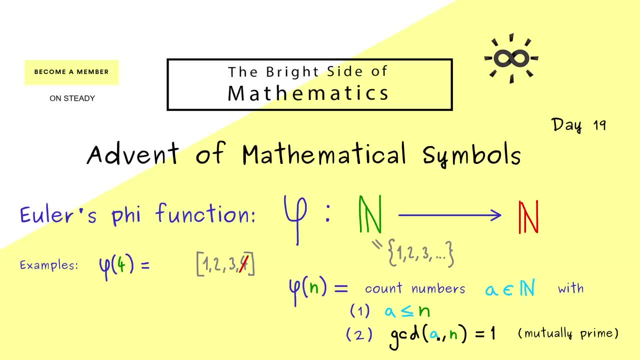 Indeed, you see, the greatest common divisor of 4 and 4 would be 4 again, not 1.. However, then you also see that 1 does not have any divisors, therefore it always fulfills both properties. Then, in the next step, we have to exclude 2, because 2 times 2 is 4.. 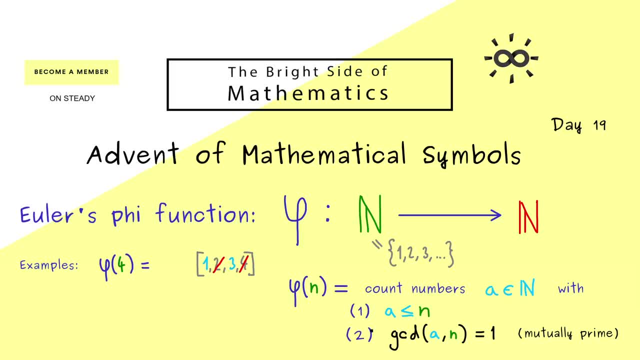 Ok, then looking at 3, we see there is no common divisor greater than 1.. And now you see, when we count the numbers that remain that fulfill both properties, we get out 2.. Hence, phi of 4 is 2.. So maybe lets look at another example. so lets choose 5..